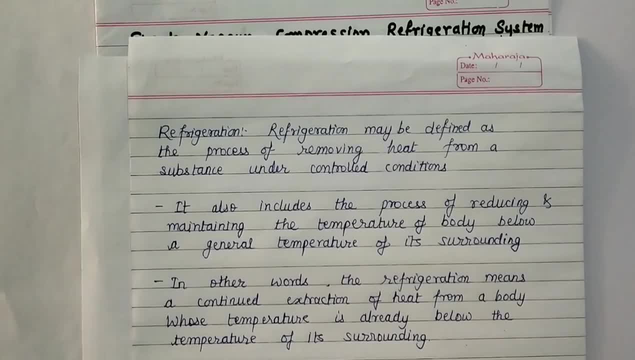 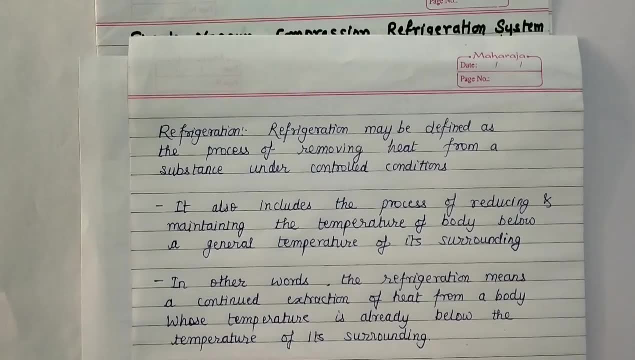 So in other words, we can say that the refrigeration means a continued extraction of heat from a body whose temperature is controlled. So this is what is done in our refrigerators also: that heat is initially extracted from a substance and that particular substance is. the temperature of that particular substance is maintained below a general temperature of its surrounding. 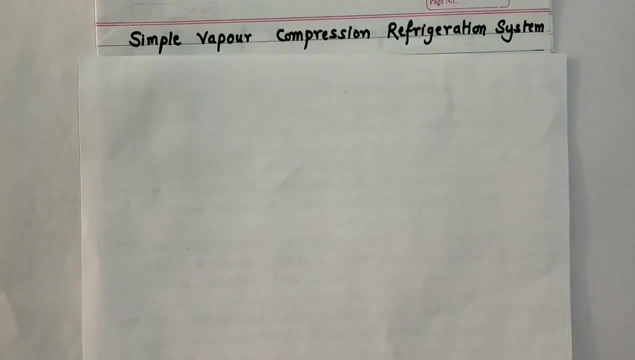 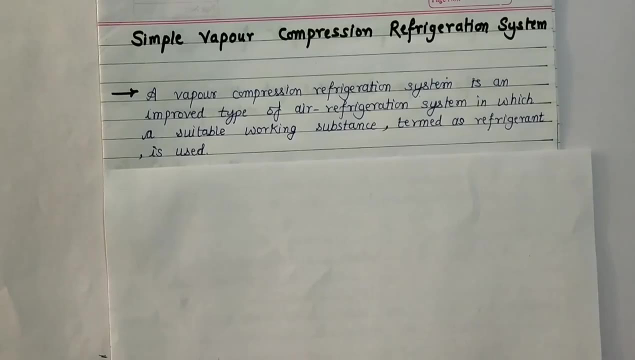 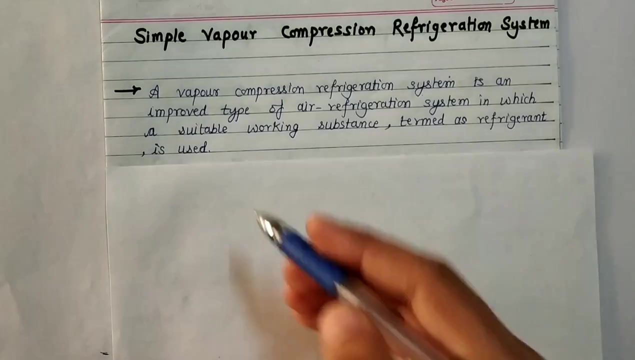 So this is what refrigeration is. Now we will go through the simple vapor compression refrigeration system. So simple vapor compression refrigeration system. So simple vapor compression refrigeration system is an improved type of air refrigeration system in which a suitable working substance, termed as refrigerant, is used. 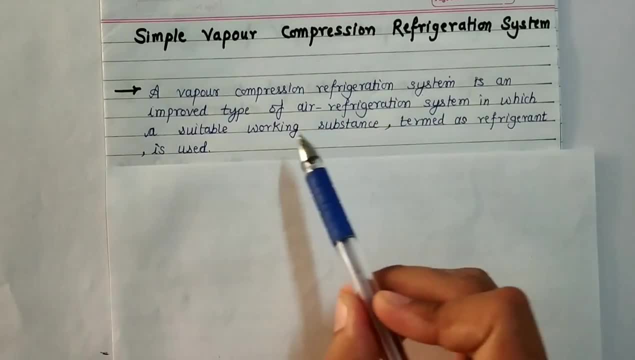 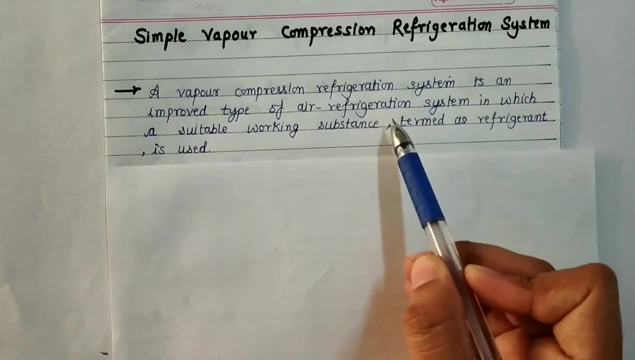 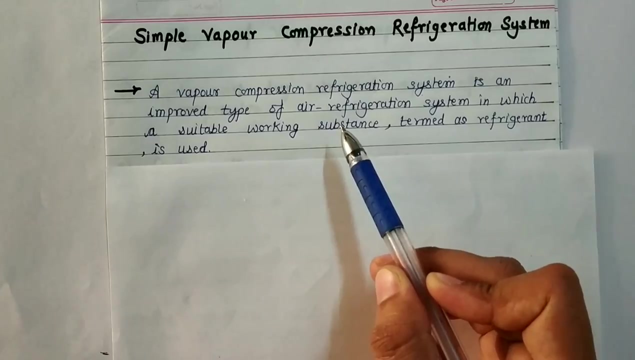 So basically, a vapor compression refrigeration system is an improved type of air refrigeration system. So air refrigeration system is a refrigeration system where air is used as working fluid or air is used as a refrigerant. Now, simple in simple: vapor compression refrigeration. 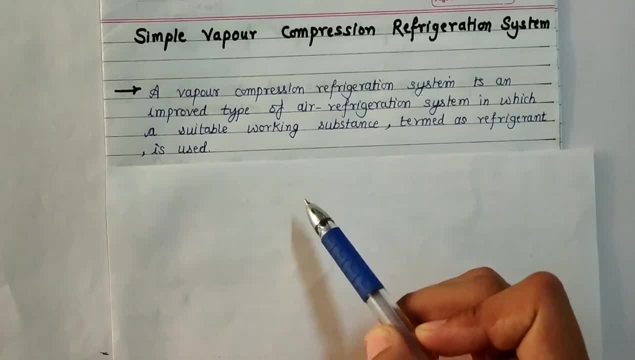 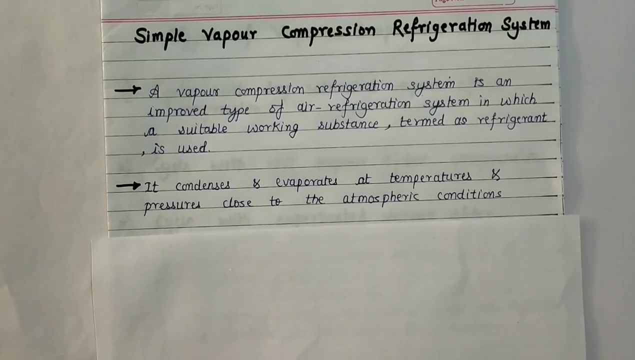 Now, simple vapor compression refrigeration system is an improved type of air refrigeration system. A suitable refrigerant is going to be used, So it may be chemical compounds fulfilling the properties required for the system. So this refrigerant then condenses and evaporates at a temperature and pressure close to the atmospheric conditions. 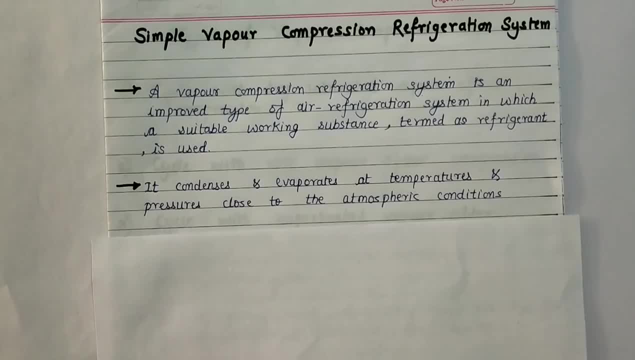 So the refrigerant is going to condense, that is, vapor refrigerant will get converted to liquid refrigerant And it is going to evaporate, which means that evaporation is going to occur, That is, liquid refrigerant is going to be converted into vapor refrigerant at temperature and pressure close to the atmospheric conditions. 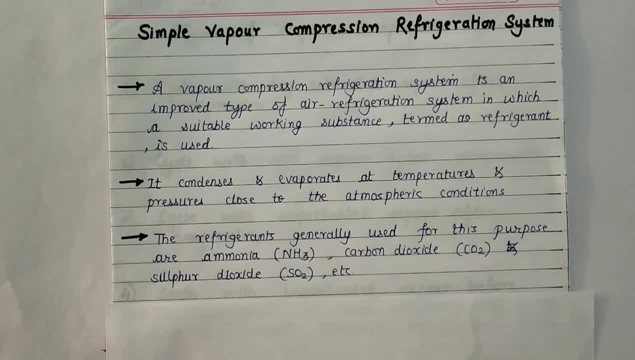 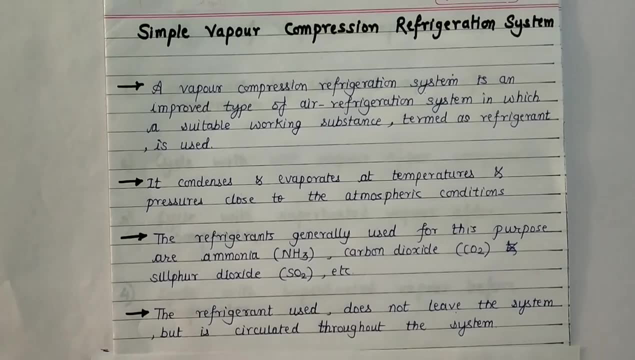 So the refrigerants which are generally used for this purpose are ammonia, carbon dioxide, sulfur dioxide and etc. So the refrigerants which are used, it does not leave the system but it is circulated throughout the system. So refrigerant will not leave the system, but it will circulate in the whole system. 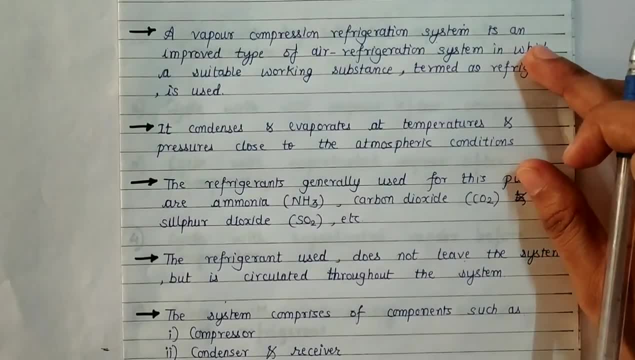 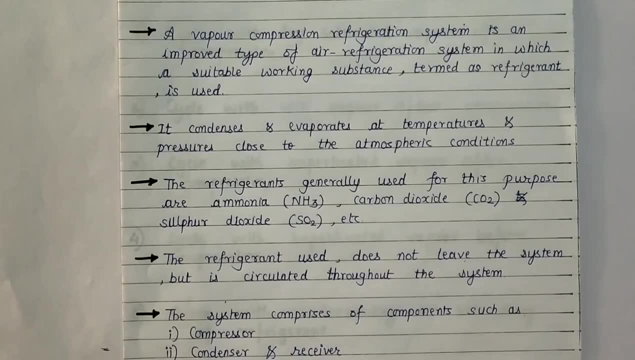 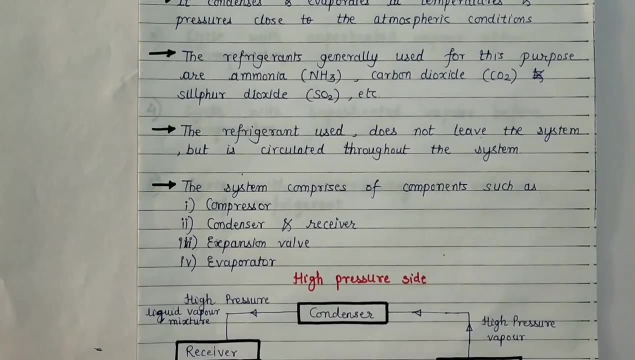 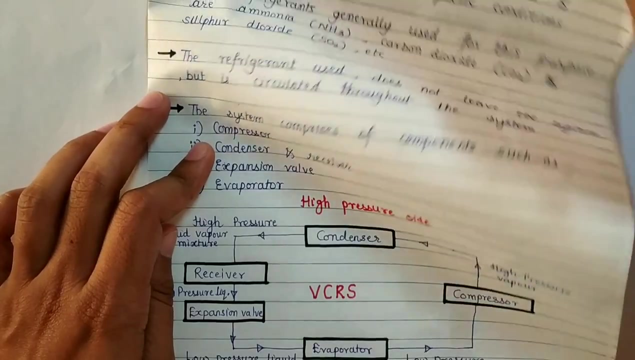 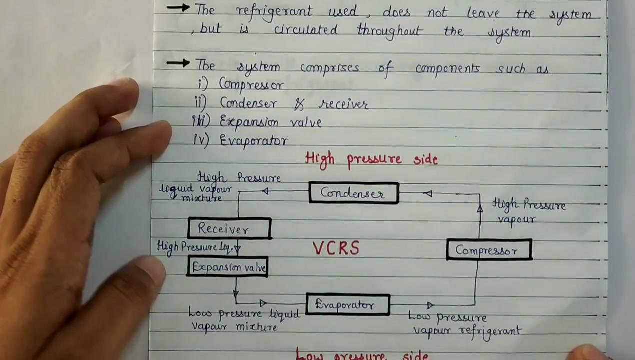 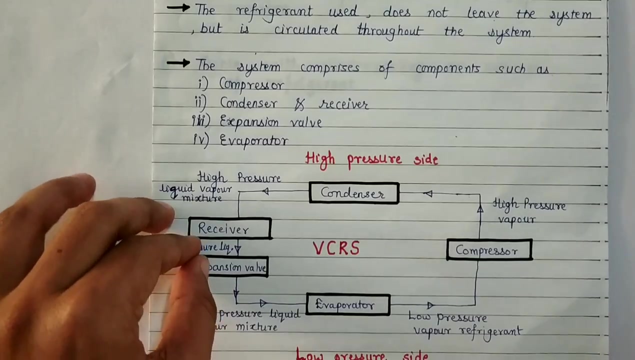 The system comprises of compressor, condenser and receiver, expansion valve and evaporator. So now we will start with the compressor. So low pressure vapor refrigerant- as you can see in the diagram, that low pressure vapor refrigerant, Low pressure vapor refrigerant, will enter into the compressor and then pressure of the refrigerant is going to increase and it will become as high pressure vapor refrigerant. 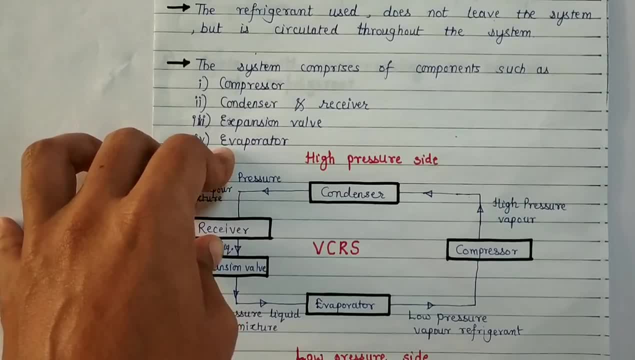 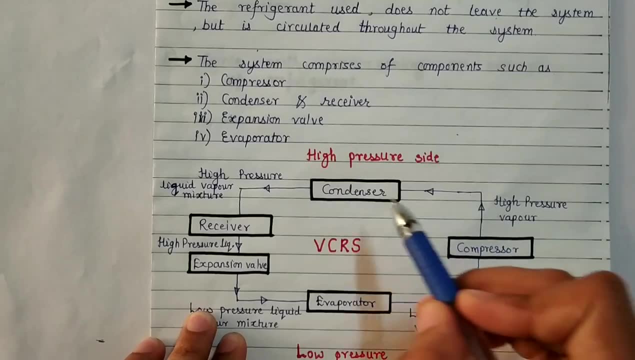 So low pressure vapor refrigerant entered into compressor is entered into the compressor and it is getting converted to high pressure vapor. This high pressure vapor then enters into the condenser And then condensation process takes place, because of which this these vapors are converted to liquid. 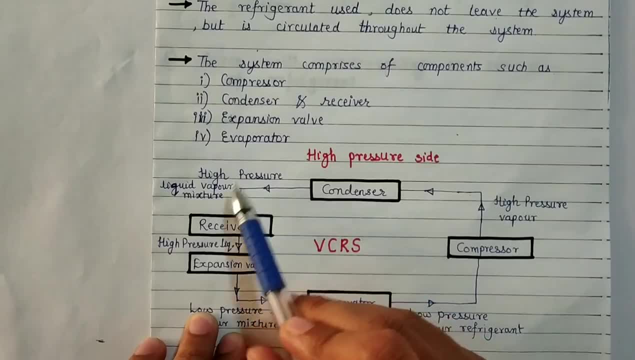 So high pressure vapor refrigerant gets converted to high pressure liquid vapor mixture after the condenser. Now, after the condenser, this high pressure liquid vapor mixture is then sent to the receiver. So receiver is basically a tank where the liquid vapor mixture is accumulated and required amount of liquid refrigerant is sent to the 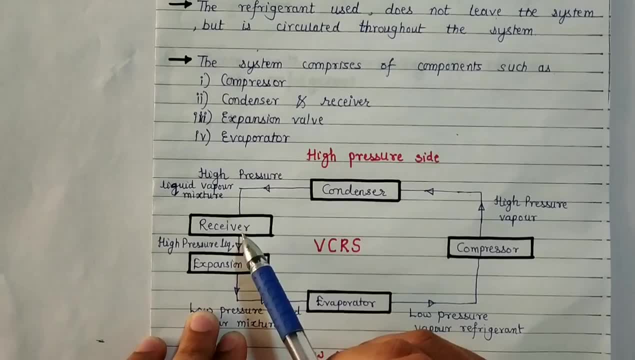 Expansion valve. so liquid amount is only going to be sent to the expansion valve, so high pressure liquid is sent to the expansion valve. now expansion valve is basically a like a throttling wall, where pressure reduction is going to take place, and also along with the temperature. 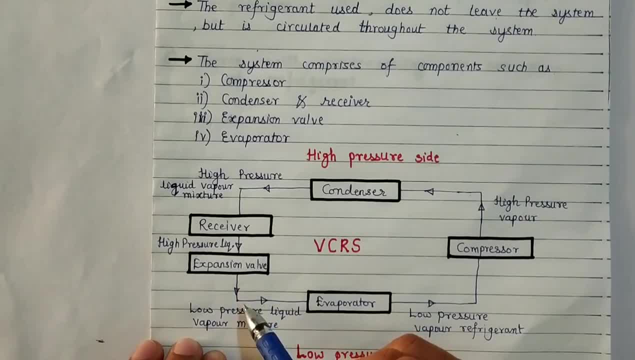 So high pressure liquid is going to be converted to low pressure liquid vapor mixture after passing through the expansion valve, that is, after the expansion. So this low pressure vapor, low pressure liquid vapor mixture is going to enter into the evaporator. so low pressure liquid vapor mixture. when entered into evaporator, so in evaporator, evaporation process is going to occur. so low pressure liquid vapor mixture will get converted to low pressure vapor refrigerant.